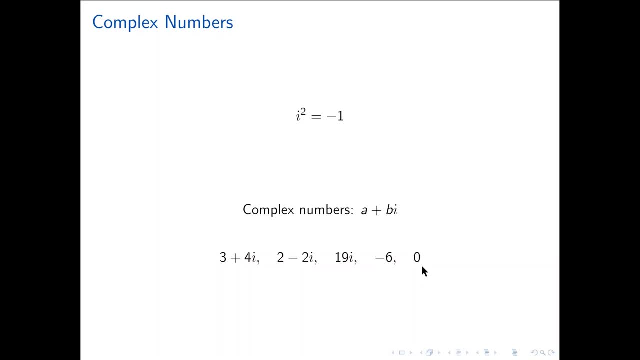 negative six and the imaginary part is zero, And zero is zero plus zero i, And you'll notice from negative six and zero, this indicates real numbers. All real numbers, in fact, are included within the set of all complex numbers, because all real numbers could just be written as whatever real 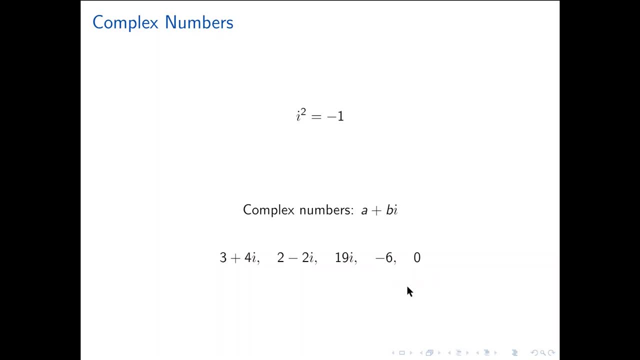 number. they are plus zero i, So complex numbers are a much broader set of numbers. All right, so we can do pretty simple arithmetic with complex numbers. If I add them together. I just add the corresponding real parts of the two complex numbers and the imaginary parts of. 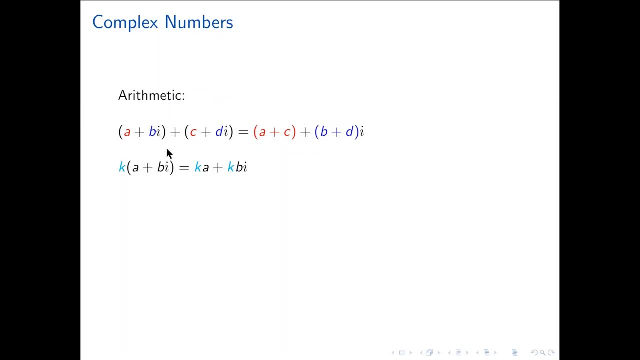 the complex numbers. So if I have a plus bi and to that I'm adding another complex number, c plus di, then the real part of the sum is a plus c, which I have in red, and the imaginary part is b plus d, which I have in blue. I can also scale complex numbers. So if I have a scalar, 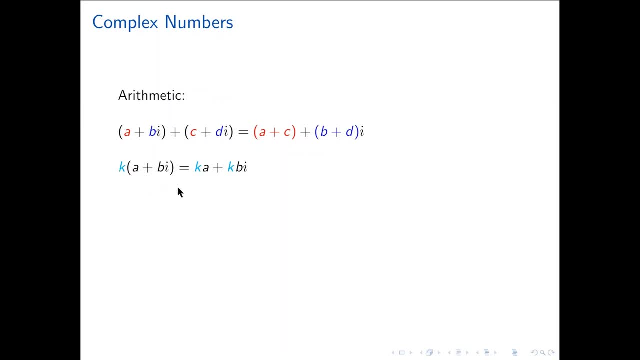 k and this complex number, then I just distribute it to the real and imaginary parts, All right, so here's an example. So I have two complex numbers in parentheses here and they're both multiplied by scalars, and then I'm adding them together. 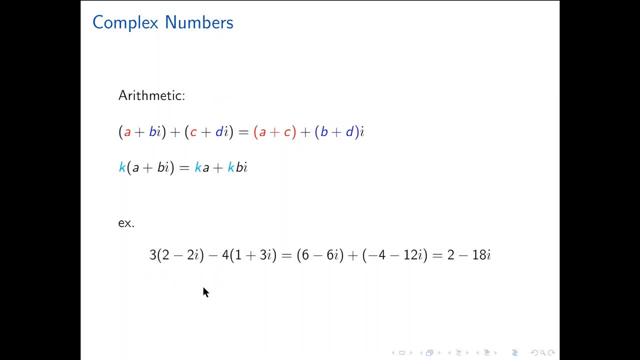 So the first thing I do is I scale this first complex number by three, and then I scale the second complex number by negative four and I get these two complex numbers- six minus six i and negative four minus 12 i, And then I add them together, So for the real parts six minus four. 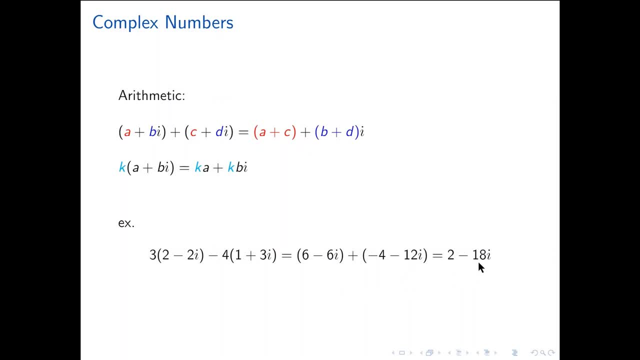 that's two, And for the imaginary parts that's two, And then I add them together. so for the imaginary parts, negative six minus 12, that's negative 18.. So this is the result. So when I multiply complex numbers, I use what you may have heard referred to as the foiling method. 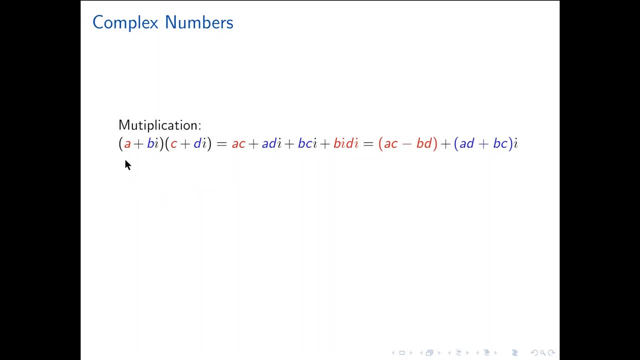 that you were probably introduced to in high school. That's where I just have two binomials, and a complex number is effectively a binomial, And I multiply the first terms, then the outer terms, then the inner terms, then the last terms, And that's exactly what we've done, right here. 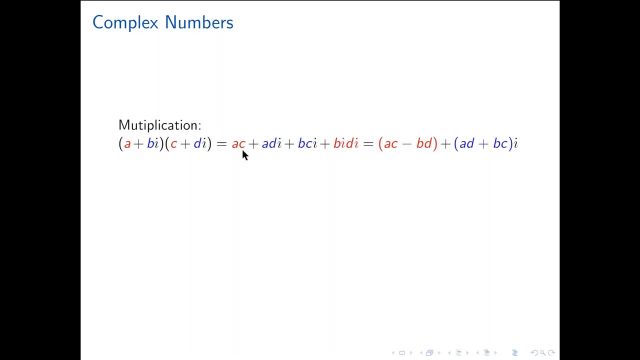 So the first terms: a times c, that's ac, and that is a real number. Then I add the outer terms: a times di, and that is this second term and that is an imaginary term because it has an i. Then I add the inner terms: bi times c, that's bci, also an. 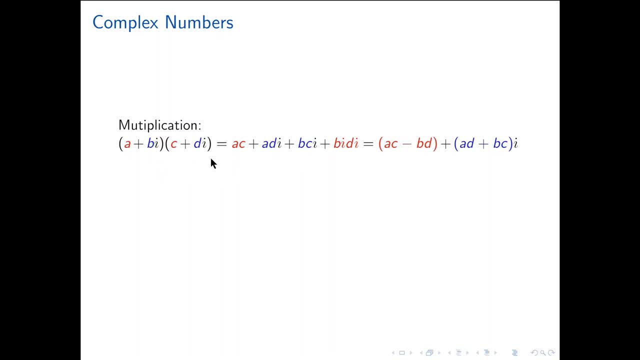 imaginary term And finally the last terms, bi times di. that's actually a real term because b and d just make bd And if I multiply both of these i's together, I get negative one by the definition of i. So actually we have two real terms- ac and negative bd, and two imaginary. 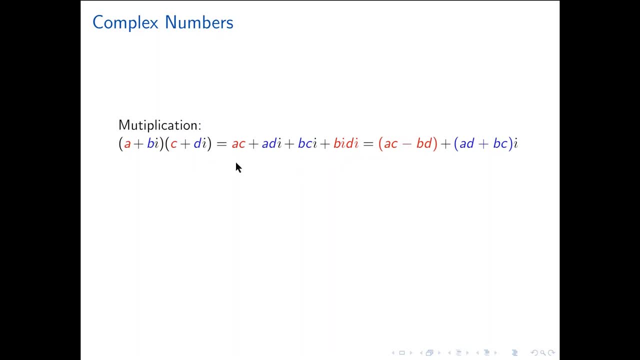 terms, adi and bci. After I find this product, the real part is ac minus bd and the imaginary part is ad plus bc. So here's an example. I'm just going to foil this out. So three times two is six. 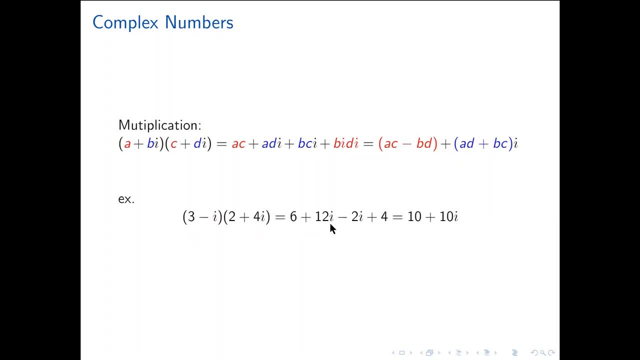 first terms. Okay, outer terms: three times four i is 12i, then negative i times two is negative two i, and negative i times four, i is four And I add the real terms: six plus four is ten and the. 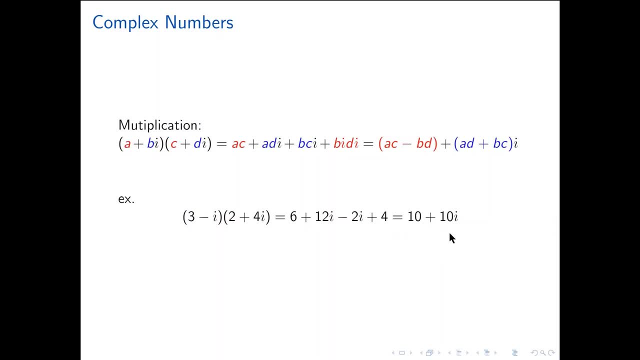 real part is 12i minus two. i is ten i and that is the product. All right, so for every complex number, which are often referred to as z, if we're just talking about an arbitrary complex number, w is also a letter that's used, okay, and that's the form: a plus bi. Then there's a special related. 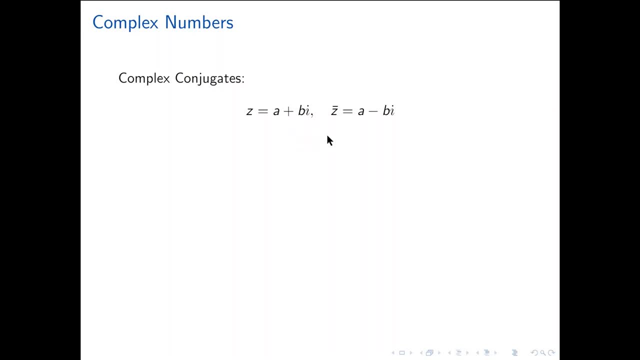 complex number called its conjugate, which I might write as z bar. okay, that's what this notation would be read as, And that is the same as z, except the sum of the two is the same as the imaginary part and the sign on the imaginary part is reversed. So if z is a plus bi, then the 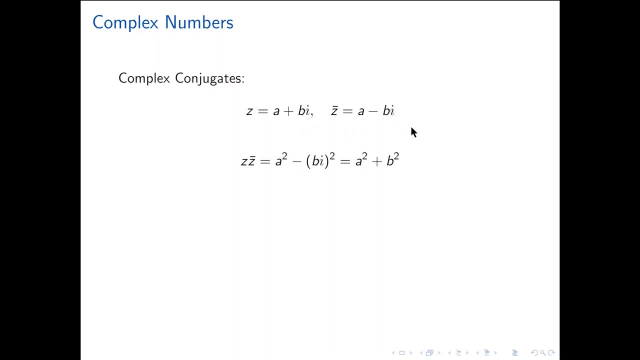 conjugate of z is a minus bi And the conjugate defines a pretty special property. If I take the product of a complex number and its conjugate, then I get a difference of squares because, again, think of complex numbers as binomials. Okay, if I had two binomials of the form a plus b and a. 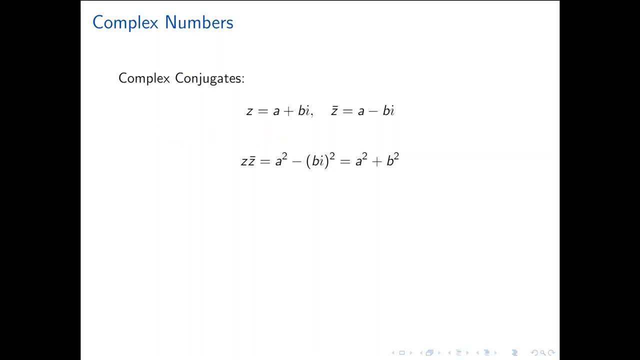 minus b and I multiplied them by one another, then we would have a difference of squares, which would be a squared minus b squared. But since we're talking about complex, it's not a squared minus b squared, it's a squared minus bi squared. Okay, we're again. 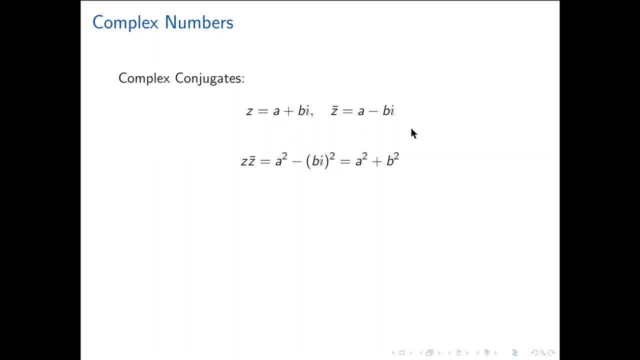 a plus bi and a minus bi are the two binomials, so to speak. So from that we get a squared plus b squared as the result, because the i squared becomes a negative one. but we're already subtracting, so this actually turns into addition, And so instead of a difference of squares, 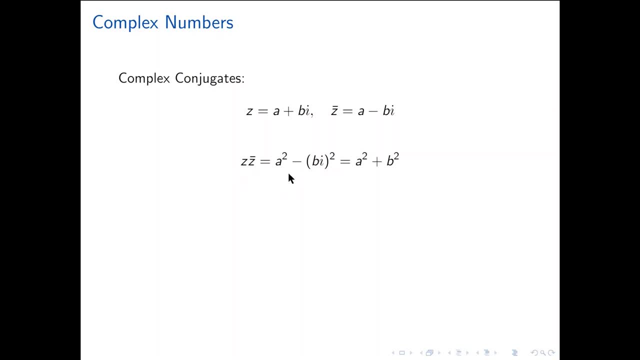 when we multiply a complex number by its conjugate, we actually get a sum of the squares of the real and imaginary parts of that number, z. So z, which is a plus bi, multiplied by its conjugate, is equal to a squared plus b squared, And you'll. 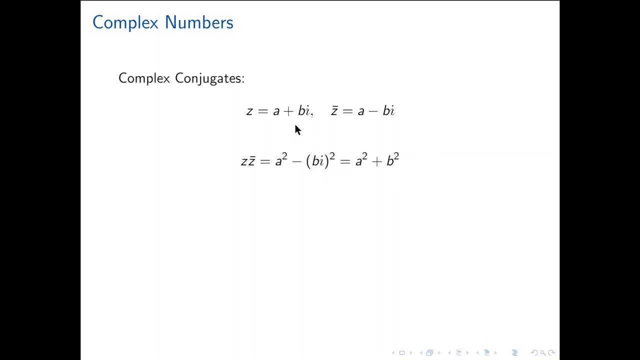 also notice that I'm multiplying two complex numbers that don't necessarily have imaginary parts that are equal to zero, but the result is a purely real number. Okay, there are no i's in this result, so a complex number multiplied by its conjugate is always purely real. 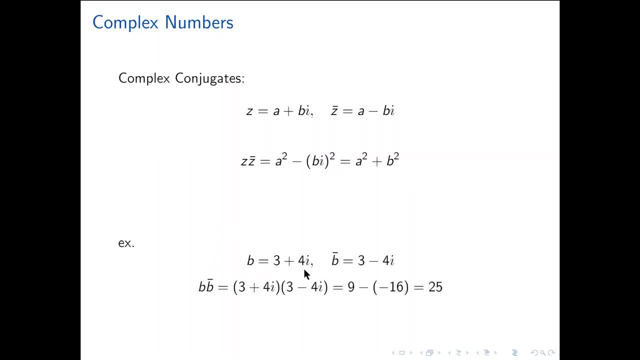 So here's an example: This complex number called b is equal to three plus four i, and its conjugate is three minus four i, And when I multiply them by one another, I get three squared minus four. i squared, so, that's nine plus sixteen, which is twenty-five. 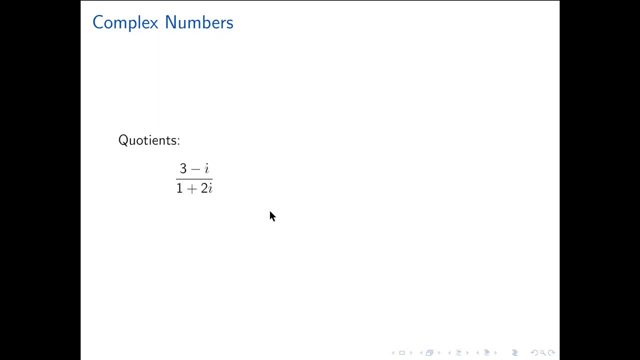 All right. so this property becomes even more useful when we're talking about quotients of complex numbers. So say, I have this quotient, just an example: three minus i, divided by one plus two i. but I'd really like to write this as just one complex number instead of writing it in this. 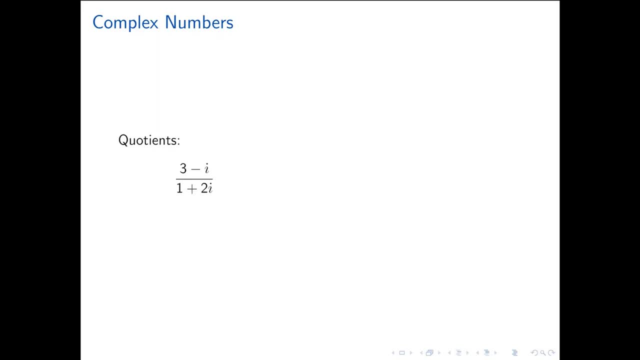 notation that indicates maybe two. Okay, well, what I'll have to do is I'll have to make the denominator of this fraction real, and the way to do that is to multiply the denominator by its complex conjugate. But of course, whatever we do to the denominator, we also have to do to the 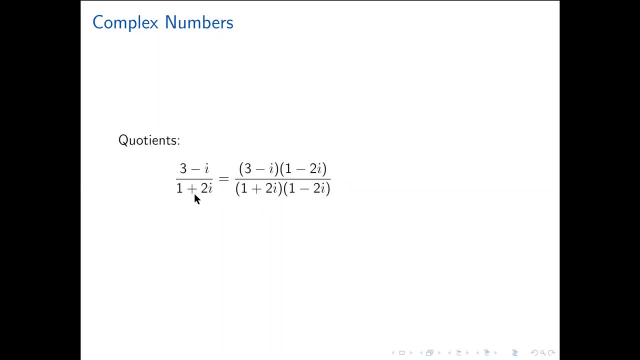 numerator, So the denominator, because it's one plus two. i multiplied by its conjugate, one minus two, i will become a real number, and that's five, and the top is just a regular product of complex numbers that we saw previously. So whatever, three minus i times one minus two, i is which happens. 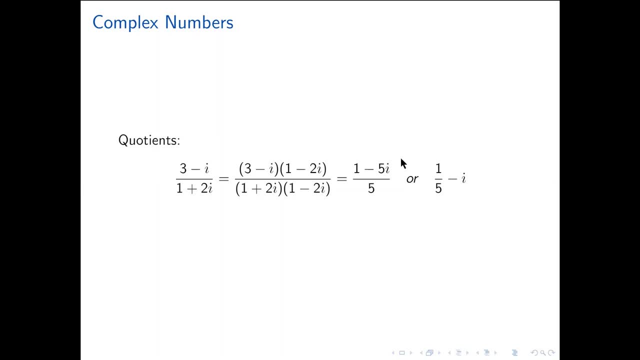 to be one minus five. i is going to be the denominator of this fraction, So I'm going to be on top, and this is just one complex number. I can write it in a better form here. more simple, I can write one-fifth minus i, and so we had a quotient here. but to make it more simple something: 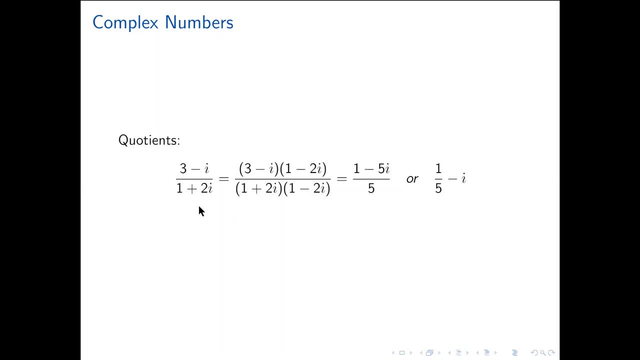 that would not have been immediately obvious. I multiply the entire fraction, the top and the bottom, by the conjugate of the denominator, and that makes the denominator real and the numerator just becomes the result of the product and I get one complex number. Okay, so let's think about the. 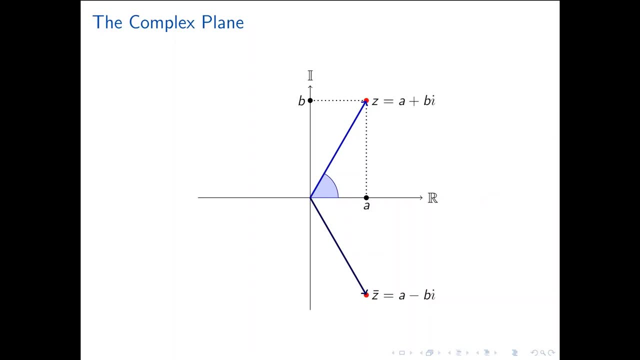 complex plane. So the complex plane is just the two-dimensional plane, where the horizontal axis is the axis of real numbers, the vertical axis is the axis of purely imaginary numbers. so complex numbers with zero real part, Okay, and all the space in between. all these quadrants contain 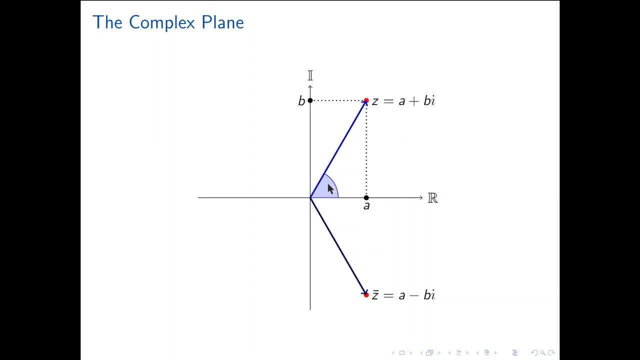 complex numbers with different real and imaginary parts, and the origin of this plane is the complex number zero plus zero i. So in that case any complex number, like an arbitrary complex number z, is plotted as a point on the complex plane where the horizontal coordinate of that point is. 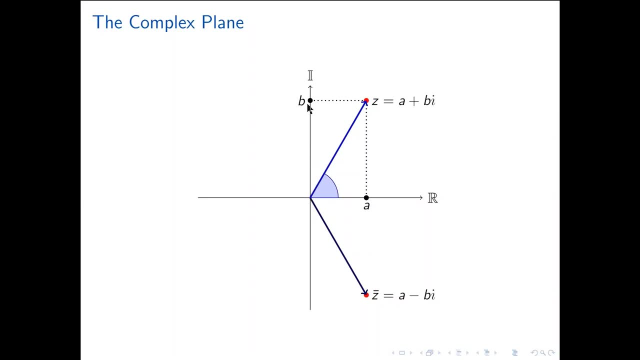 the real part a and the vertical coordinate of that point, that complex number is the imaginary part b. So if z equals a plus bi, then its coordinates are a, comma, b, so to say, and z's conjugate is going to be reflected about the real axis because the real parts are the same. a is the 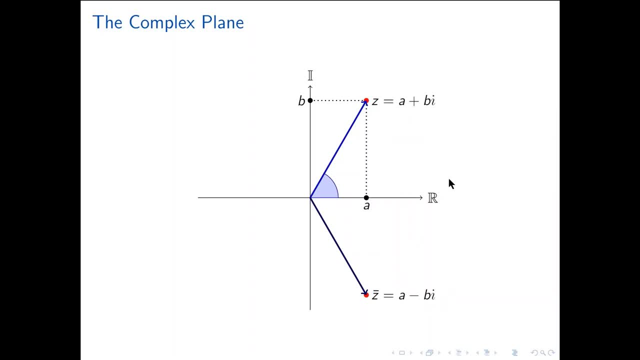 same for both of these, but the conjugate of z has negative bi instead of plus bi. so the imaginary part has been reversed and so the point gets reflected about the real axis. So we can also think about the length of the distance from the point representing a complex. 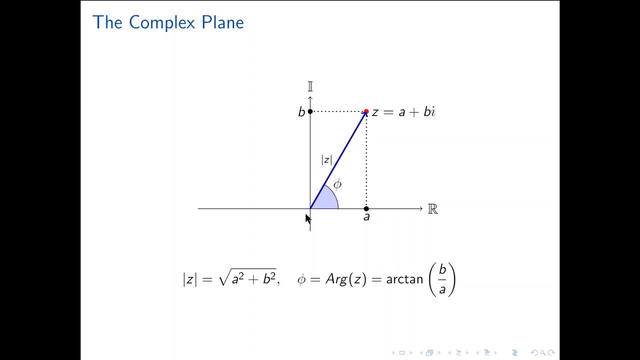 number on the complex plane to the origin of the complex plane, which is zero plus zero. i all right. and that distance is not called the magnitude, like it would be for a vector. it's called the modulus of a complex number which I write, as in this case, for a complex 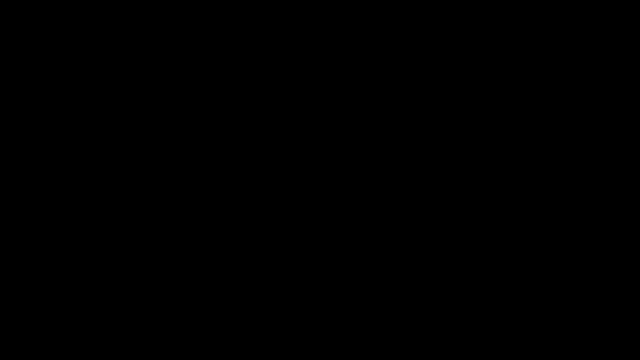 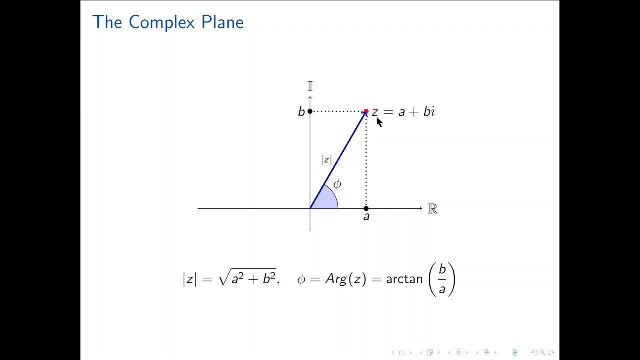 number z. it would be z in between these two vertical bars And the angle that the line from the origin to the point on the complex plane for z makes with the real axis. okay, this angle, phi, is called the argument of z, And so the way we find the modulus is just by the distance formula. it's the square root of the. 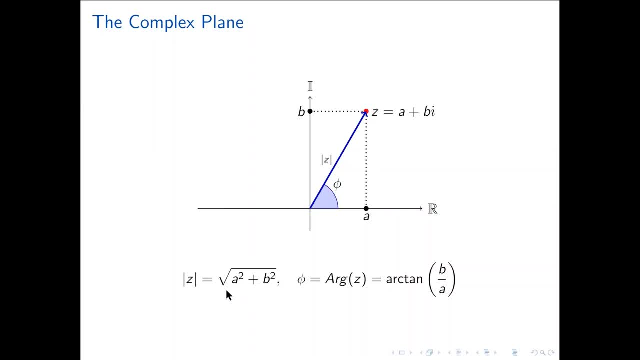 horizontal distance squared plus the vertical distance squared, which is right here, the square root of a squared plus b squared, and the argument phi is equal to the arctangent of b over a. All right, so we can also write complex numbers in polar form, which is pretty straightforward. 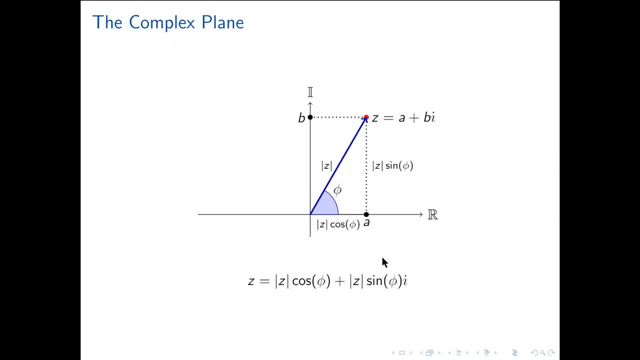 we just write their real and imaginary parts not as their own numbers, like five or negative three, but in terms of the modulus and argument. So this horizontal distance, which is also a, is also the modulus of z times, cosine of phi, the argument. 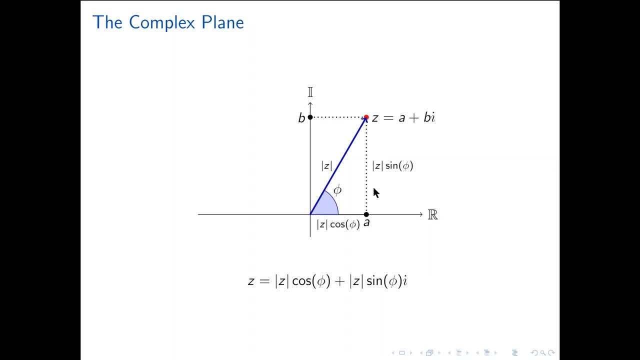 and this vertical distance, which is b, is also the modulus of z times sine of phi, And so z is equal to a plus b i, or the modulus of z times cosine phi plus the modulus of z times sine phi times i. So let's take a moment to talk about Euler's formula, which is as follows: 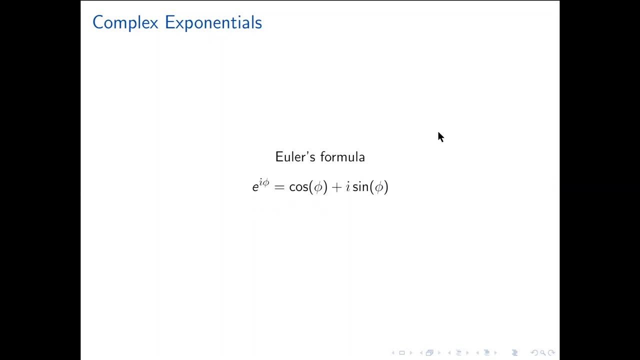 e to the i phi is equal to cosine phi plus i sine phi, and this is related to the polar form of a complex number, as we'll see. So, prior to this formula's introduction there was no definition, essentially, of what a complex exponential would look like. 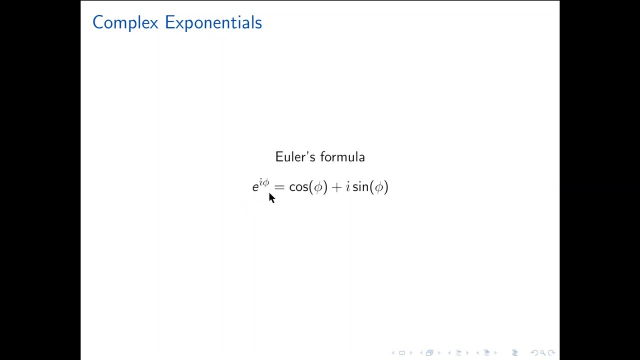 and that's what this is called. A complex exponential is e to any complex power, essentially. So in this case we can look at this formula and it's saying that a complex exponential is a complex number, and if that's the case, then it implies that a complex number 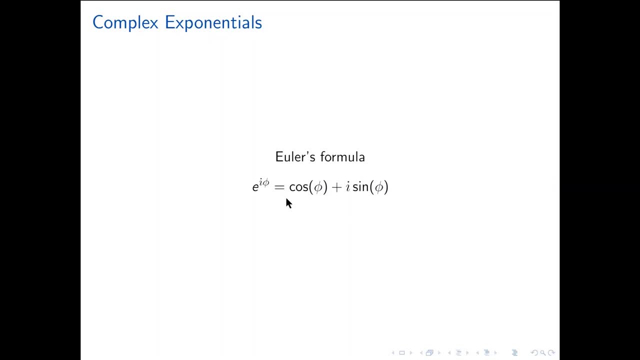 could be rewritten as a complex exponential. I mean cosine phi plus i sine phi. that is awfully similar to the polar form- I'll go back- which we have right here- of a complex number, z. It seems like phi might be an argument of some sort, and if i were to 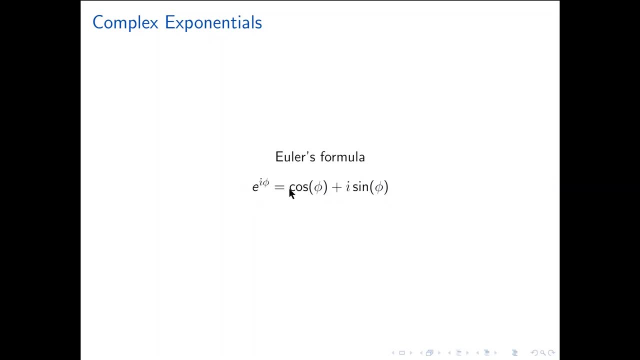 multiply this complex exponential by some quantity, then that would multiply cosine phi and i sine phi, which is very similar to how the modulus of z multiplies cosine phi and i sine phi. And so let's look at this example here. So again, an arbitrary, complex number z. 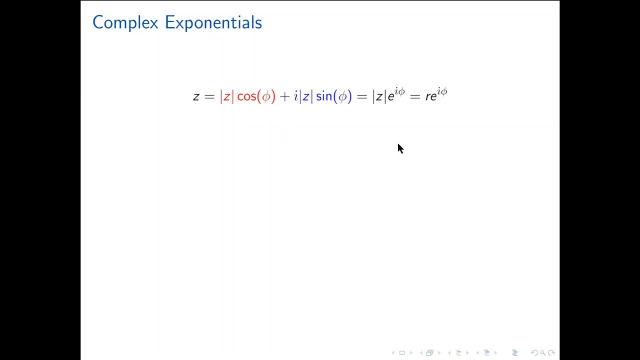 and this is the polar form. And what you'll notice is, if Euler's formula says that e to the i phi is equal to cosine phi plus i sine phi, then the modulus of z times e to the i phi is equal to the modulus of z times e to the i phi. And so what you'll notice is, if Euler's formula 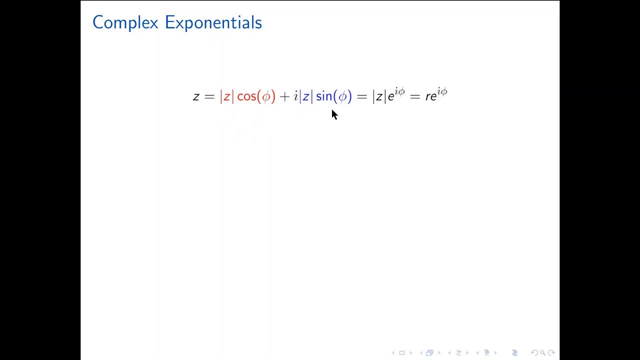 says that z times cosine phi plus the modulus of z times i sine phi. So in other words, Euler's formula says that if i have a complex exponential, then the exponent, the part that isn't i, is the argument, and the coefficient in front of the complex exponential is going to be the modulus. 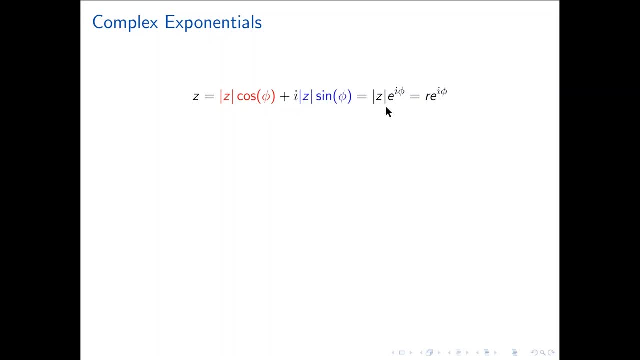 of the complex number that has been written in this exponential form, And so we usually write this coefficient in front. We just call it r. So here's an example: I have a complex number, z, and that's 1 minus i, And so if I want to rewrite z in exponential form, then I'll have to go. 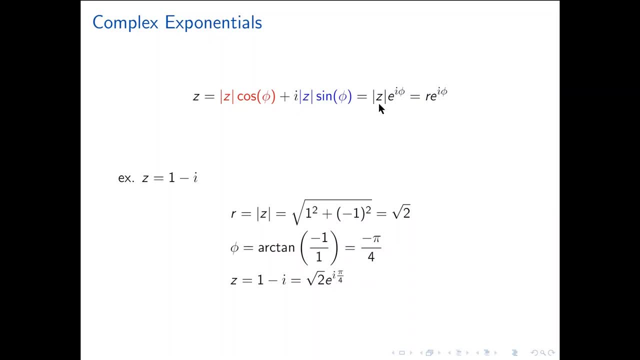 through these steps. First I'm going to have to find r, which is the modulus of z. So the modulus is just calculated through the distance formula. So I take the square root of 1 squared plus negative 1 squared, and that is root 2.. And then I want to find the argument, So that's the arctangent. 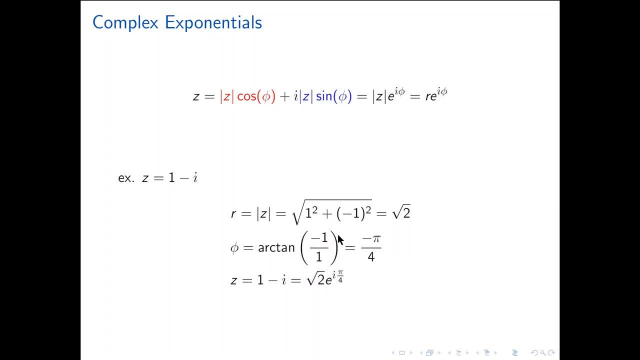 of the imaginary part over the real part, arctangent of negative 1 over 1.. And that is negative pi over 4.. So now I know r, the modulus root 2.. I know phi, the argument negative pi over 4.. And so z in exponential form is equal to root 2e to the i pi over 4.. 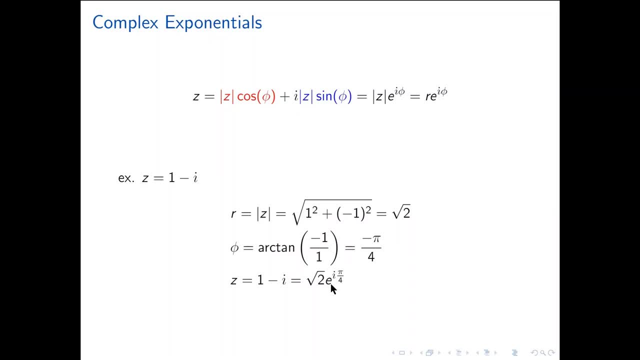 And again, let's see what this would look like if it were expanded out. So first the e to the i, pi over 4 part, when expanded by Euler's formula, is going to look like cosine of pi over 4 plus i sine pi over 4.. But both of those terms are multiplied by 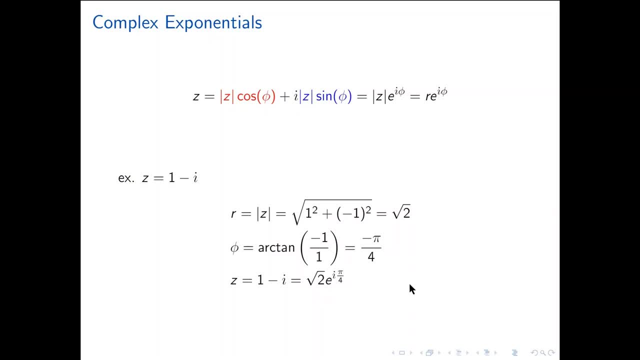 root 2.. So it's going to be root 2 cosine of pi over 4, plus i times root 2 sine pi over 4.. And that is exactly the polar form of this complex number. But you can also just find it from the: 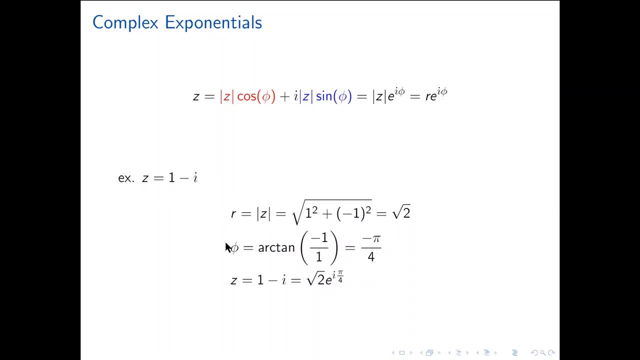 regular form of the complex number. like we did here, We find the modulus, we find the argument and then we replace r and phi in r e to the i phi with the actual values of the modulus and argument. Okay, so here's another example: a complex number, w, and that is negative, 2 plus 3i. 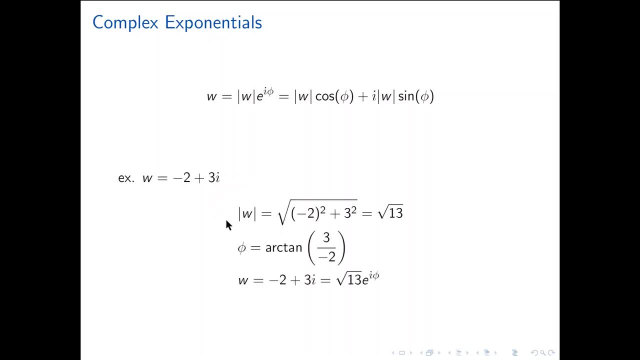 So we're going to go through the same steps. Find the modulus, okay, the square root of the real part squared plus the imaginary part squared, and that is root 13,, the argument which is the arctangent of the imaginary part over the real. 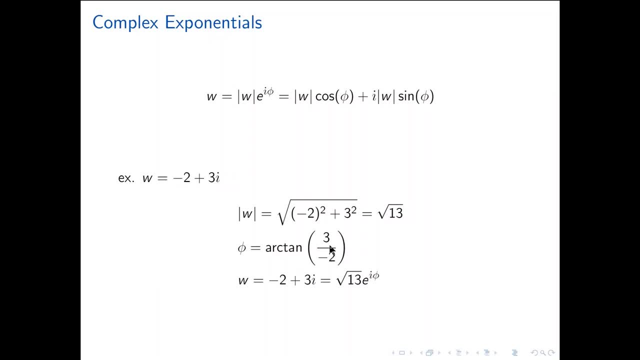 part, And since the arctangent of 3 over negative 2 is not some clean value, we'll just understand in the final answer that phi is equal to whatever the value of this arctangent is, And so in that case w is equal to negative 2 plus 3i, and in exponential form it's equal to. 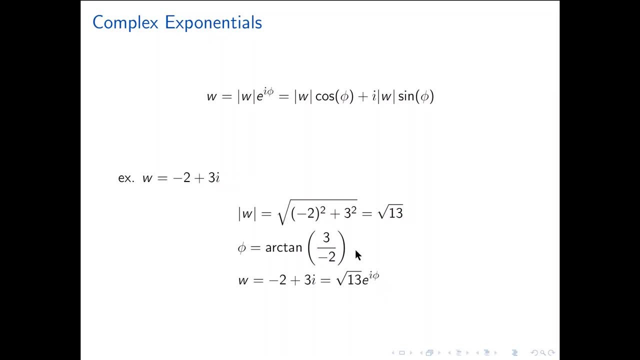 root 13. Times e to the i phi. where again, phi is this value of the arctangent. All right, so now let's think more generally about raising e to the power of any complex number, with some real part and some imaginary part. Before, when we were looking at e to the i phi here, 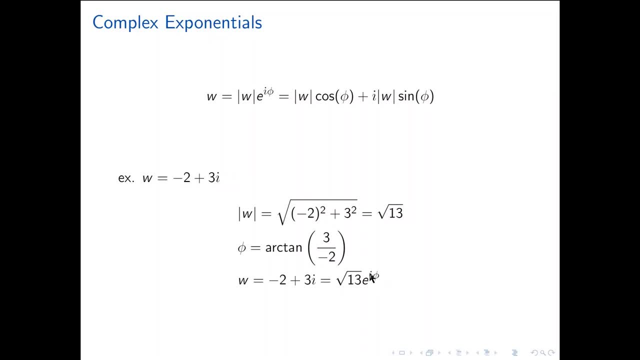 this is technically raising e to a complex power, but the real part of this is zero, right? This is zero plus phi i. So now let's actually look at raising e to powers of complex numbers in general. so I have a complex number alpha, and that is e to the a plus b i. a plus b i is a complex number. 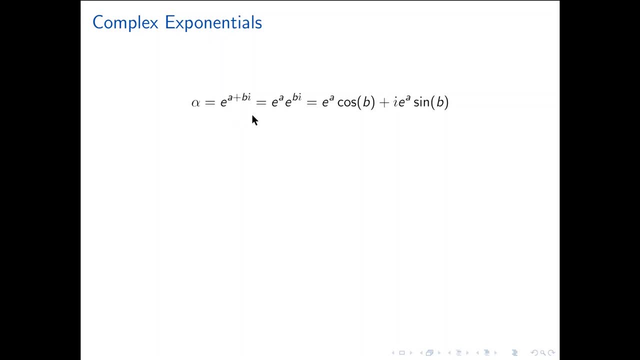 And so by the properties of exponents, I can rewrite this as e to the a, times e to the b i. all right, And so by Euler's formula, e to the b i is equal to cosine b plus i sine b, and both of those terms are multiplied by whatever's in front, which is e to the a. 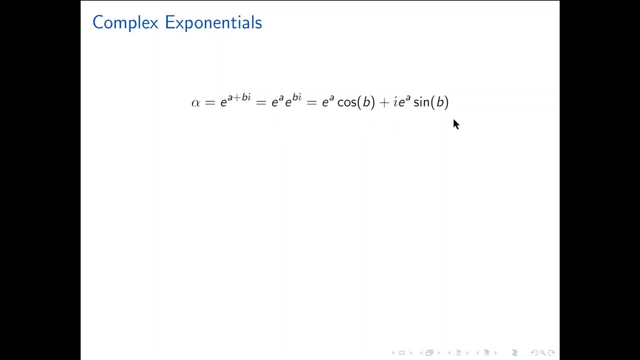 So in total it's e to the a cosine b plus i, e to the a sine b, And we'll get a little bit of a difference here, because we're going to take the number of exponents- e to the a cosine b plus i, e to the a sine b, And what you'll notice is that we're not going to 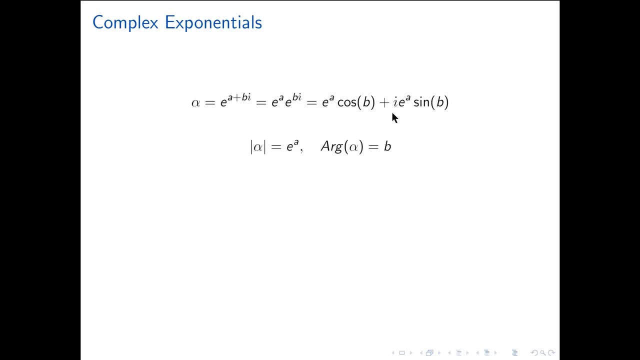 we're not going to take the number of exponents e to the a cosine b, but we'll take the number of exponents. is that if this were the polar form of a complex number, then B would be the argument of that complex number? and what are we multiplying both of these cosine? 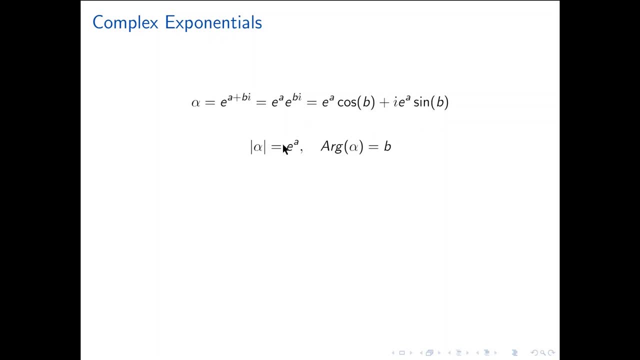 and sine terms, by e to the a. so e to the a would serve as the modulus of this complex number. so if I have a complex exponential with a complex number of the form a plus bi, then the modulus of that complex number is e to the a and the. 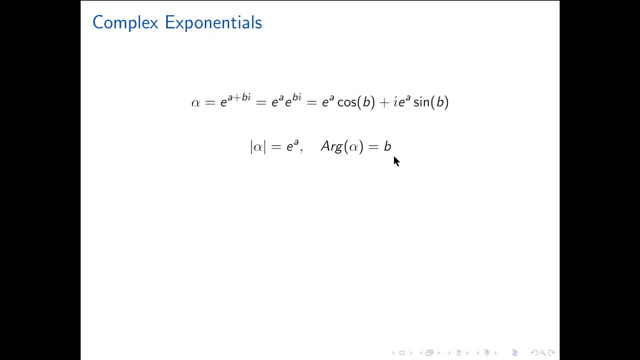 argument of that complex number is B. so here's an example. I have a complex number which is e to the 1 plus pi over 3 times i, and so first thing I'm going to do is split up that exponential into e to the 1 or just e times e to the pi. 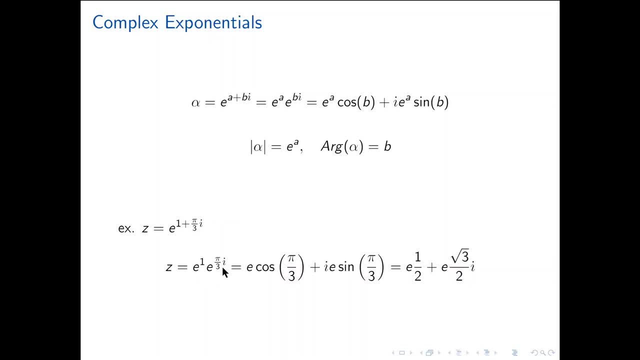 over 3 times i. alright, and so by Euler's formula e to the pi over 3, i is equal to cosine pi over 3 plus i sine pi over 3. I multiply both of those terms by e which we see here, and conveniently enough, of course, this example was chosen for this reason, pi. 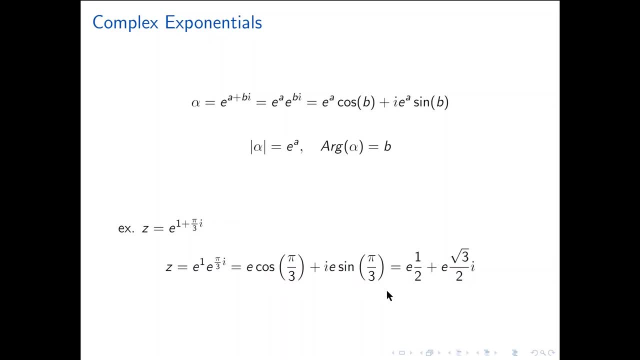 over 3 allows us to simplify cosine and sine into 1 half and root 3 over 2, and so the result? the answer is e times 1 half plus e times root 3 over 2 times i. so we take a complex exponential and now we rewrite it as a regular complex. 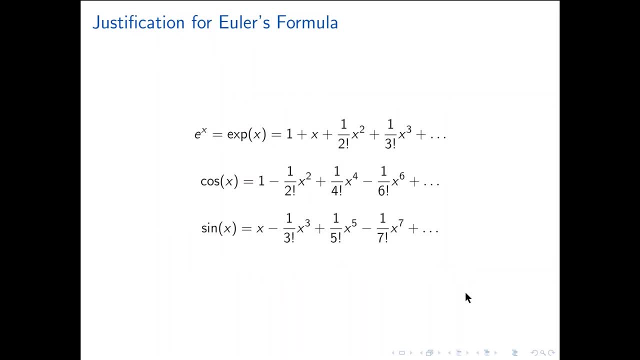 number in this form that we saw before. alright. so Euler's formula, even though it is technically a definition- and definitions can be somewhat arbitrary- needs some justification to maybe understand why there's reasoning behind it. because there is. so first I want to introduce a notation. so if we have e to the x right, that's just an exponential. 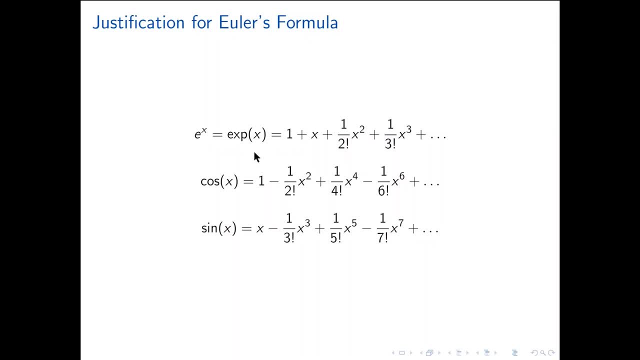 but we can also think of e to the x, or the exponential of x, as it's sometimes called, as a function of x. I mean, that is what e to the x is, but if I'm thinking about the infinite series representation of e to the x, and you also see the 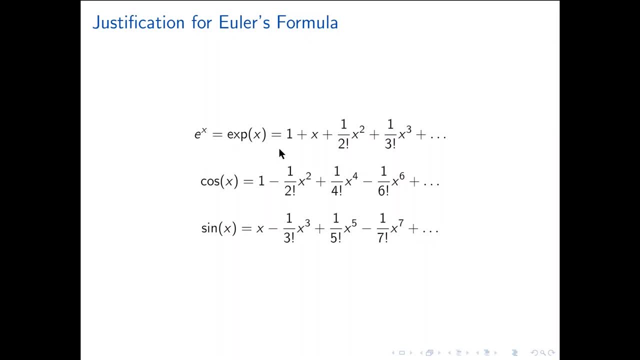 infinite series of cosine and cosine of x, and you also see the infinite series of cosine and cosine of x, and you also see the infinite series of cosine and cosine and sine. okay, then we're talking about an infinitely long polynomial, and so we might not think of that intuitively as being e to the power of x, and so another. 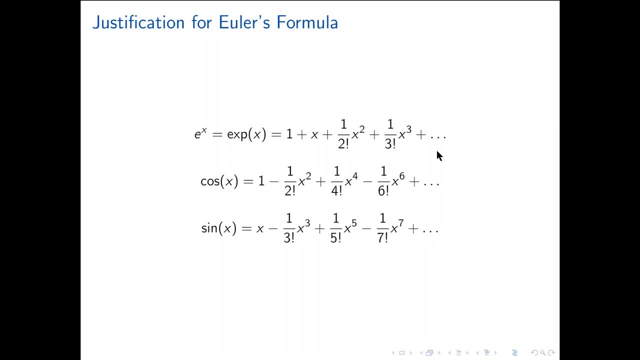 notation is just to write: exp of x. this is the Taylor series from calculus. this is the infinite series of cosine of x and the infinite series for sine of x. alright, so now let's say that we're looking at the infinite series not of e to the x, but the exponential of i phi. so instead, 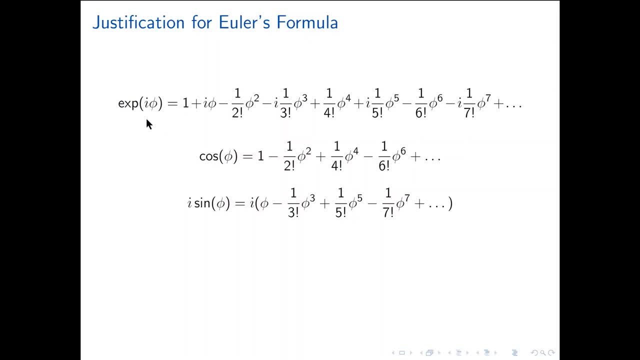 of x. we're just having i phi. how does that change things? well, I'll go back for a moment. the infinite series was originally 1 plus x plus 1 over 2. factorial x squared plus 1 over 3. factorial x cubed plus 1 over 4. 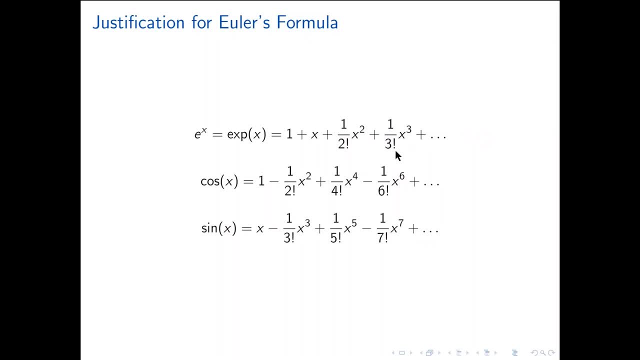 factorial x to the fourth and so on. you know, we just increment the factorial on the exponent for every term. so in this case, instead of 1 plus x plus 1 over 2 factorial x squared, we have 1 plus i phi minus 1 over 2 factorial phi squared. and 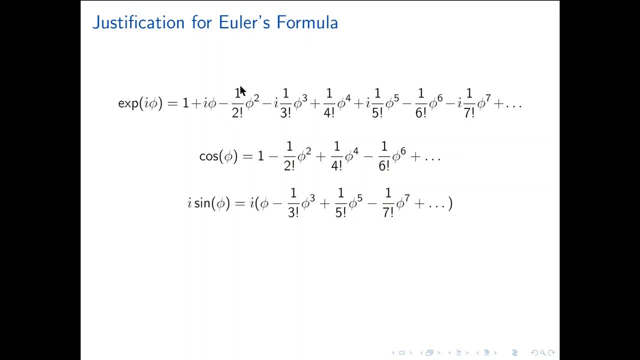 what? where did we get this, this subtraction, from? well, this was originally one over two factorial times: phi, i squared, but the i squared becoming became a negative one. then for the next term, we're multiplying it by another phi and another i, and so the i just goes to the front. all right, and then this is one over four. 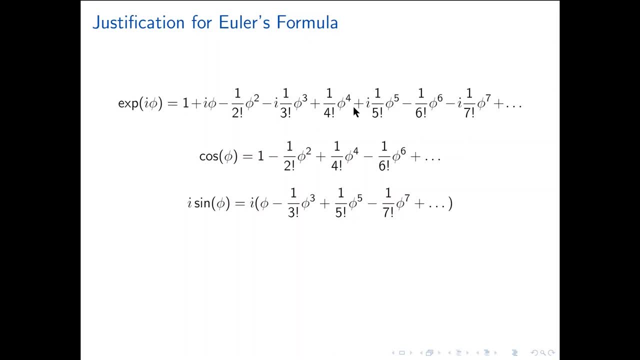 factorial times: phi i to the fourth and i to the fourth is just one, so that's why we're just adding one of this term and there's just phi to the fourth and so on, and so you can hopefully glean a kind of pattern out of this. we have plus one, plus i phi, and then we have minus, minus, plus plus. 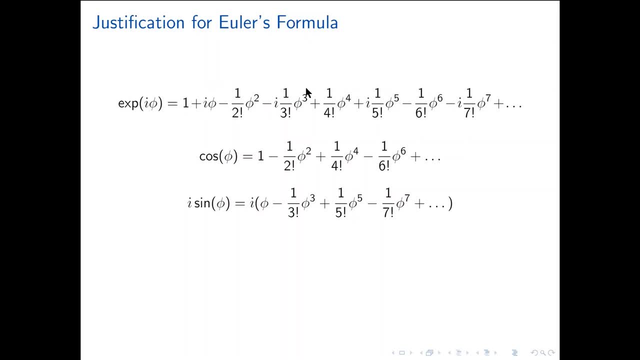 minus, minus and so on. so the pattern basically alternates. we have two additions and two subtractions, and then two additions, and so on for every term in the infinite series. for the exponential of i phi, how about just cosine of phi? well, this is the exact same infinite series as. 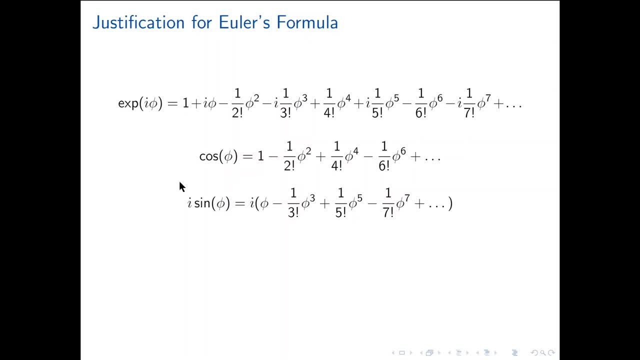 that for cosine of x, just with phi. and what if i looked at the infinite series of i times sine of phi? well, in that case, i'm just multiplying the infinite series of sine of phi you by i. and what does this tell us? well, this shows us by the infinite series, that euler's formula 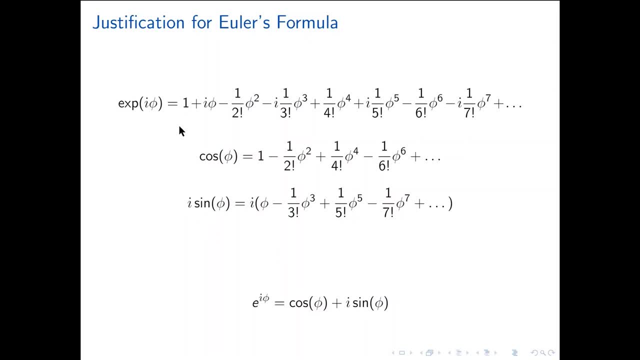 is true that it makes sense. and why is that? well, let's look at the terms of the exponential of i phi. the first term is one- and where could we get a one from? how about the first term of the series for cosine of phi? and then our next term is i times phi. that second term comes from the series. 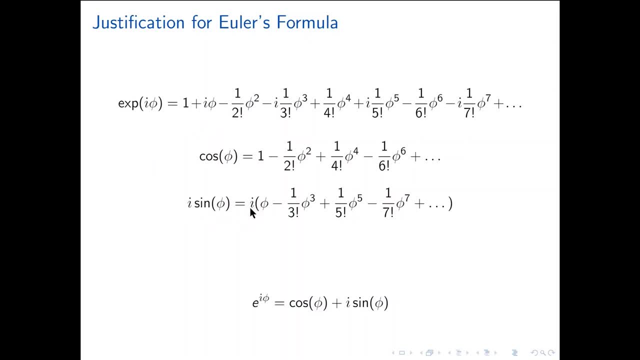 of i times sine phi, because that is i- is being applied by all the terms in this series and the first term of the series is phi. so the first term of the entire thing is i phi, and then the next term is minus one over two factorial times phi. 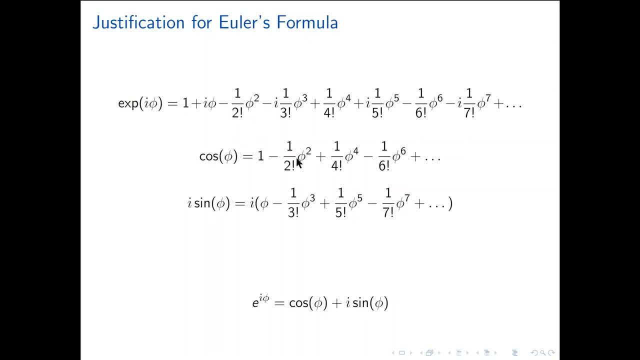 squared, and that's exactly the second term in the series for cosine of phi. and so it seems like if i alternate picking terms from first cosine of phi and then for the series of i times sine of phi and so on, i in fact construct the exact series for the exponential of i times phi, and that is true. 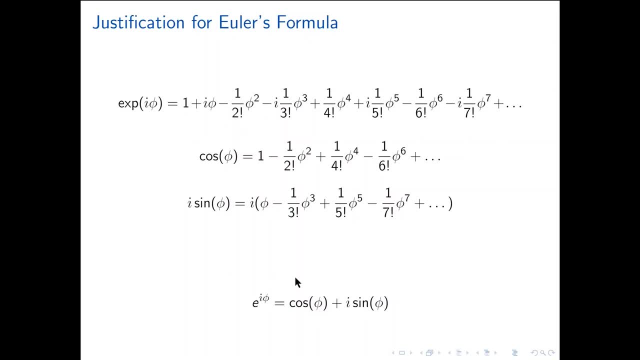 that is a pattern that we see, and so this formula that e to the i phi is equal to cosine phi plus i sine phi, is justified by the infinite series of these functions. so now that we understand euler's formula, let's look a bit more at the implications of 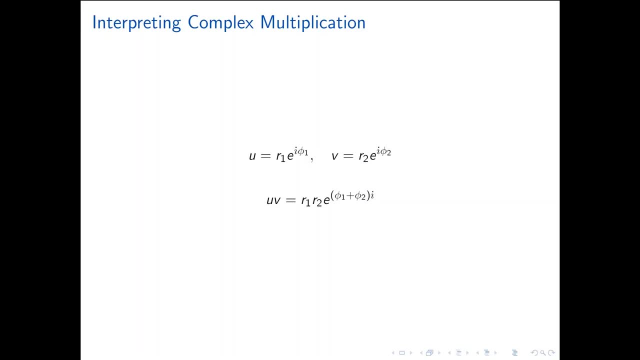 complex numbers written as complex exponentials. so if i have two complex numbers, u, which is equal to r1 times e to the i phi 1, and v, which is equal to r2 e to the i phi 2, then when i add these together i get the formula that e to the i phi 2 is equal to cosine of phi. 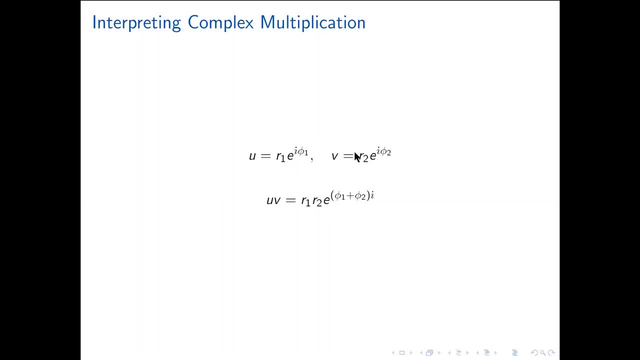 i obviously get this. i multiply r1 and r2 together in front of e and i add the exponents. but what is this telling us about the complex numbers, perhaps in the complex plane? well, whatever coefficient we have before the exponential, r1 and r2 in these cases, are being 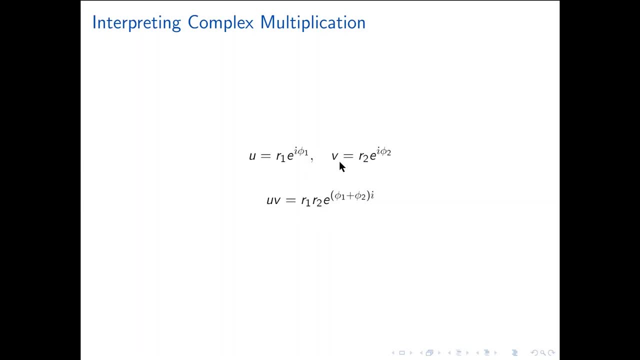 multiplied by each, by each other. but those are also the moduluses of u and v respectively. so it seems like when i take the product of two complex numbers, what i'm doing in the complex plane is i'm multiplying the two complex numbers by the modulus of the two moduluses of the operands. 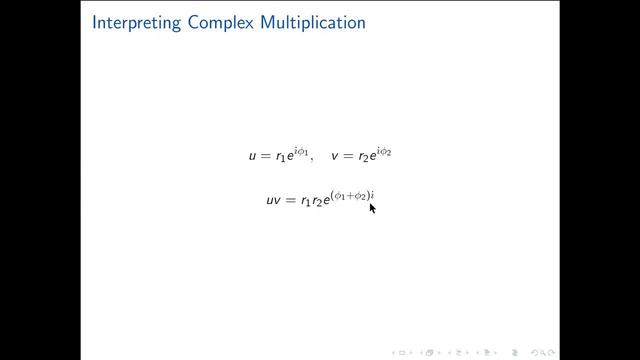 here. and what do i do with the arguments? i add them, i add the arguments. so let's look at an example. so let's say u is equal to 2 e to the i, phi over 6, and v is equal to 3 halves e to the i. 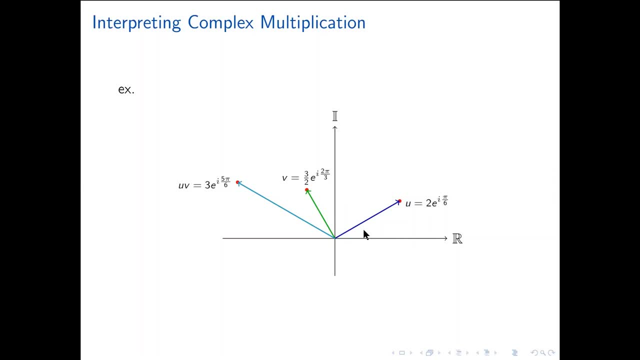 2 pi over 3, so i multiply the moduluses. so the modulus for the length of u is 2 and the length of v is 3, halves the product of those is 3 and in fact the length of u is 2 and the length of v is. 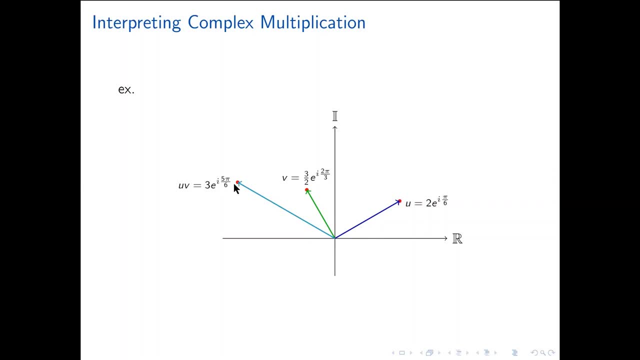 3 and in fact the length of the product uv is 3, as we see here. how about the arguments? well, i am adding the arguments. look at the angle of the blue arrow and the angle of the green arrow and hopefully you can put together visually that the angle of the cyan arrow is the sum of those two. 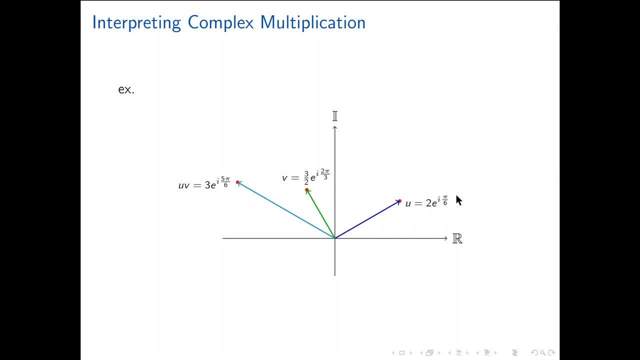 but we can also look at the formulas of these. so the argument of u is pi over 6, the argument of v is 2 pi over 3, which is 4 pi over 6, and the argument of their product is 5 pi over 6, which. 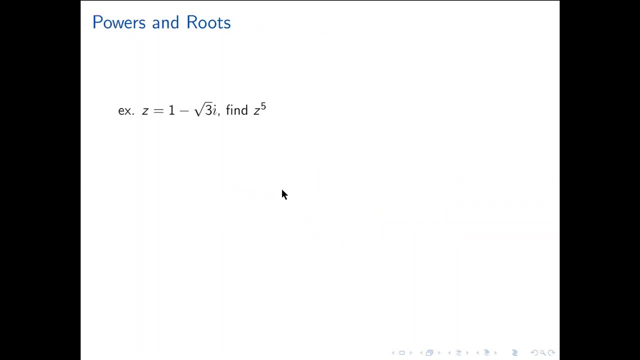 is 4 pi over 6, and the argument of their product is 5 pi over 6, which is 4 pi over 6, which is 4 pi over 6. okay, so now we're going to talk about powers and roots of complex numbers. so here's an example: i. 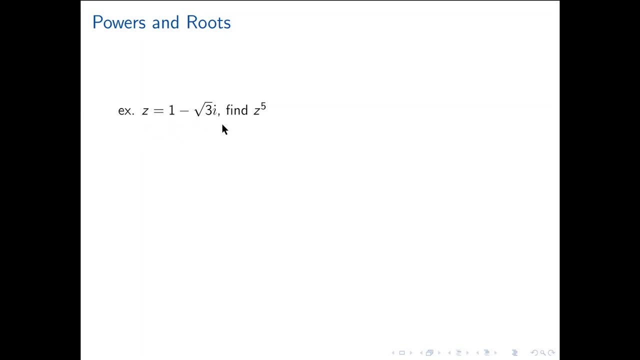 have a complex number, z, that's 1 minus root, 3 times i, and i want to find what z to the fifth is. so what would be really useful is to convert this complex number to a form where raising it to a power is just simple and straightforward. how about the exponential form? so let's do that. let's first 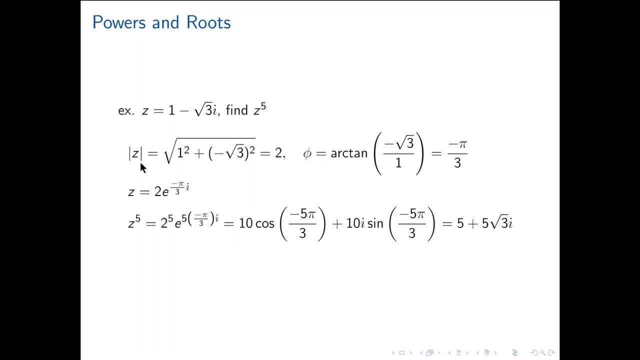 convert it to the exponential form. so i find the modulus, that's the exponential form, and i'm going to write that as the square root of the real part squared plus the imaginary part squared, and that's 2, then phi, the argument is the arc tangent of the imaginary part over the real part, that's. 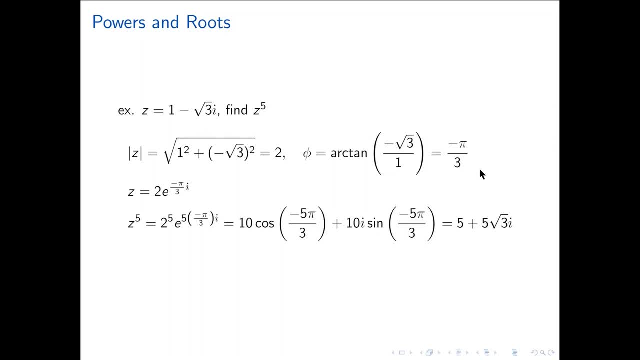 negative pi over 3, and so i put those two together and i get the exponential form, which is 2 e to the negative pi over 3 times i. all right, and so now that i know the exponential form of z, i'm going to raise it to the fifth power. so z to the fifth is 2 to the fifth times e to the 5 times negative. 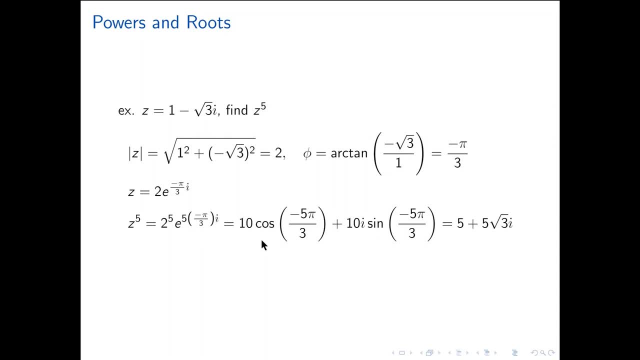 pi over 3, i. and now i can write the exponential form of z to the fifth power, and i'm going to write this in polar form, or expand this exponential by euler's formula, if you will. and so 2 to the 5th is 10, so both of these terms are multiplied by 10 and i have this. 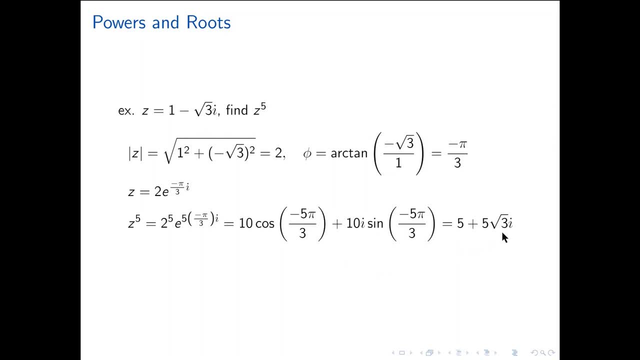 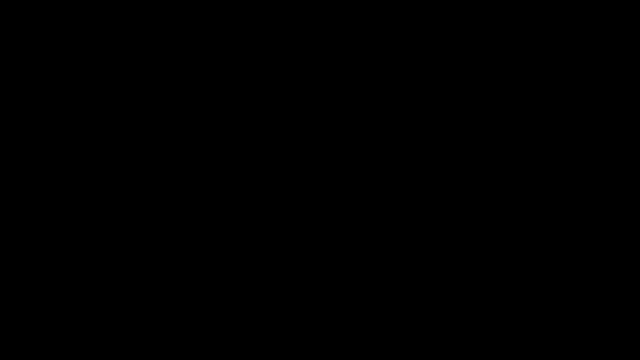 cosine and this sine and it happens to reduce to 5 plus 5 times root 3 i, and so if i want to write this in polar form, i'm going to write this in polar form and i'm going to raise this quantity to the nth power. what i'm also doing is i'm raising what it's equal to to the. 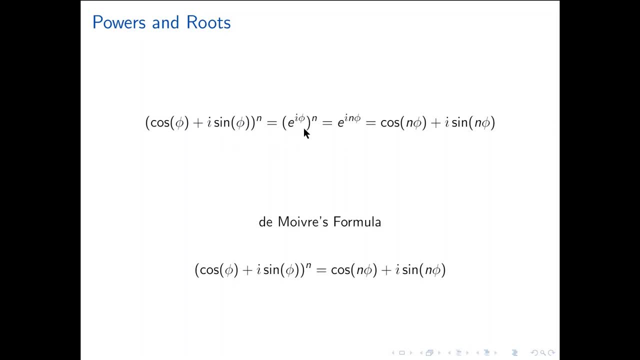 nth power and it's equal to by euler's formula: e to the i phi, e to the i phi to the nth power. this is equal to e to the i n phi, just by simple exponent properties. and now by euler's formula, i rewrite this as a more standard, uh complex number, and that is: cosine of n phi plus i times sine of. 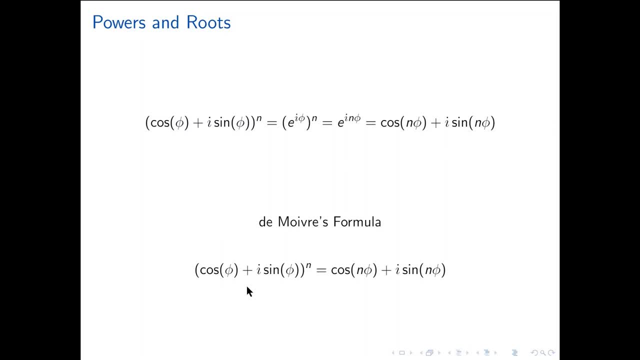 n phi. and so de maverick's theorem says that cosine of phi plus i sine phi to the nth power is sine of n phi plus i sin of n phi. okay, so we talked about powers, but let's talk about roots. so we know, perhaps from the quadratic formula or just from intuition, that 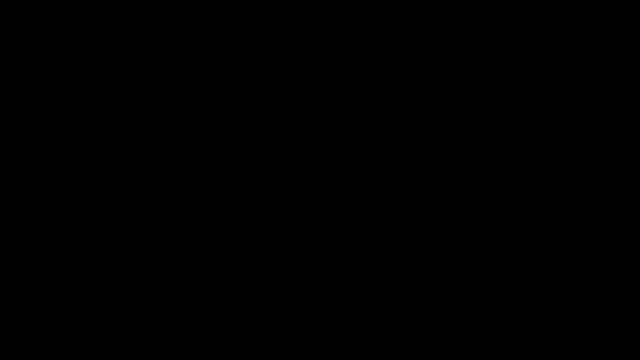 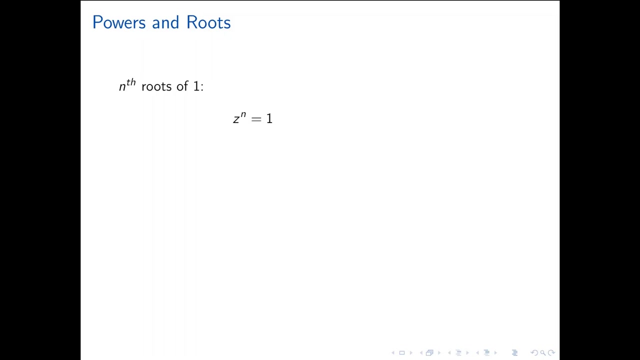 if i have a number and i want to find its roots, but i also have complex roots to worry about. in fact, if i'm taking the nth root, then i have n complex roots which include the real roots, which include the real roots, which include the square roots, which include the 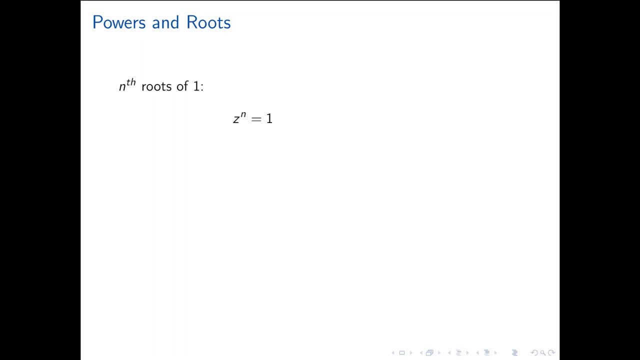 roots of that number that i'm taking the nth root of, and we'll see that in a moment. so let's say i have complex numbers, or of the, which are z, and when i raise them to the nth power i get one. so the nth roots of one are these complex numbers, z. so what are they? well, z is a complex number again. 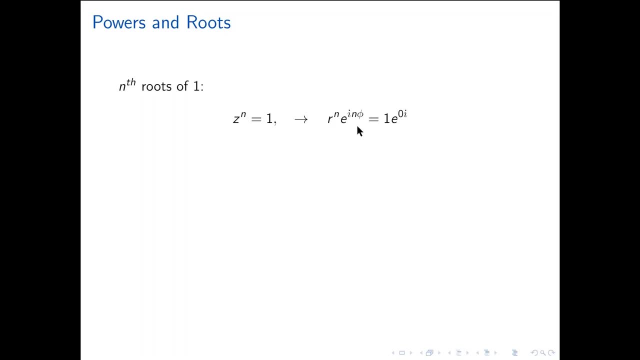 which can be written in the form re to the i phi. and so if i'm raising it to the nth power, then i have r to the n times, e to the i n phi. and what if i wrote one which is complex, number one plus zero i as a complex exponential? well, that would be one e to the zero i. and so what's interesting? 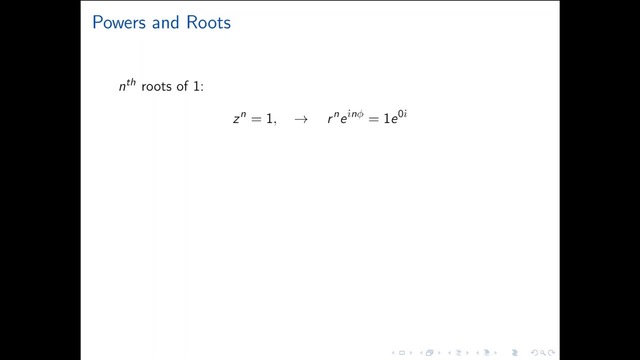 is, and this becomes apparent just from looking at the complex plane and sort of using intuition. i'm not going to prove it, but two complex numbers are equal only if their moduluses are equal and their arguments are equal, and so in this case, what i'm saying is that 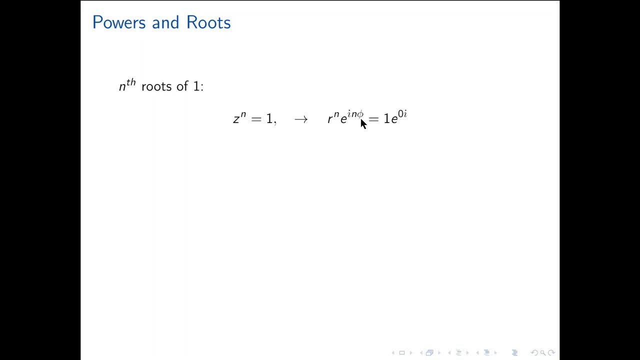 r to the nth power is a complex number, and so if i raise it to the nth power, i get one. r to the n must equal one and i n phi must equal zero i. so let's first talk about r to the n being equal to one. so in that case, pretty simply, r needs to equal one, right one to any power equals. 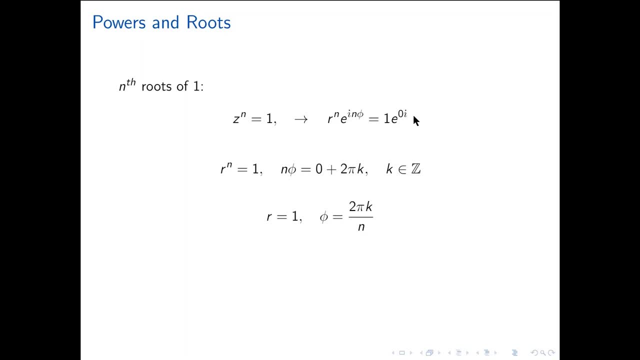 one. well, how about the exponents being equal? so they both have i in them, right, i n phi and zero. i both have i in them, so i can get rid of that. and so i have n. phi is equal to zero. but what's this? plus two pi times k, what does that mean? well, think about the unit. circle on the unit. 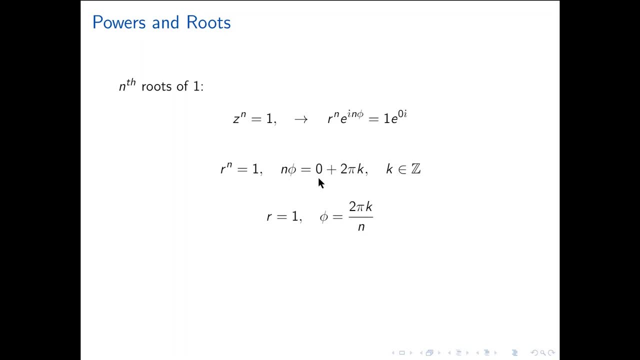 circle, we have a unit circle and we have a unit circle and we have a unit circle and we have a. i have a point, but in this case i'm specifying arguments here. zero is the argument. but if i go a full revolution around the circle, if i go a full angular distance of two pi radians around that, 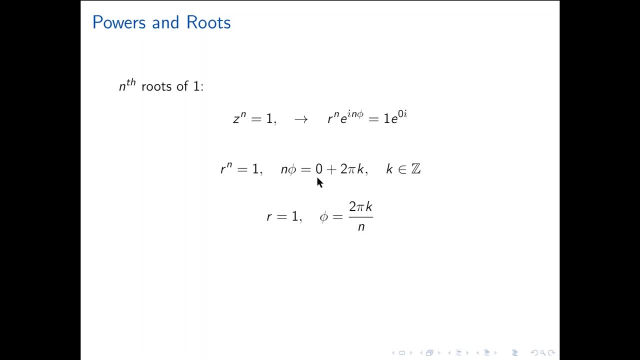 circle, i arrive back at the same argument, effectively. and so if i take the argument zero or i add on to it any integer multiple of two pi, and that's what k is, k is any integer, it could be negative, five zero, one right, and so, um, if i add any integer multiple of two pi onto zero, i go around the circle once and 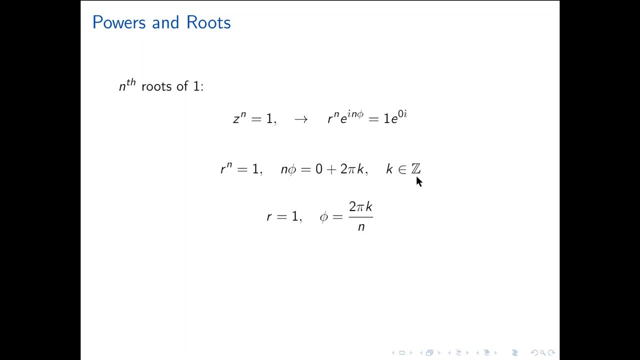 i arrive back at the same argument. and so, right here, this notation basically just says that k is a member of the set of integers. if i solve for phi, now right, i already know that r is one. if i solve for phi, it's equal to two, pi k over n, where k is some integer. and again, just think about going. 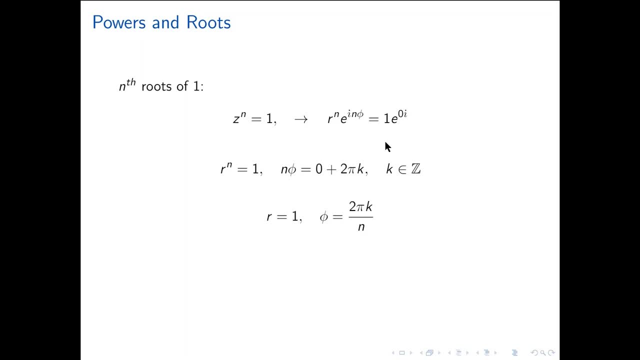 around the circle, some integer multiple of two pi radians, and you arrive back at the same argument, which is zero, and we can use this to find what the roots of one are, which are the complex numbers z and so in that case, these complex numbers are going to have a modulus of one, which is r, and they're going to have an argument of two. 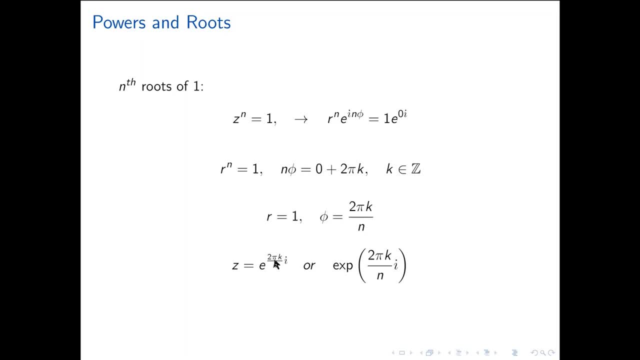 pi k over n, where k is some integer and that exponent is multiplied by i. and here's the exponential function notation that we can use, because you know writing fractions in an exponent is kind of a tricky thing to do. and so z is equal to the exponential of two pi k over n, and so that's. 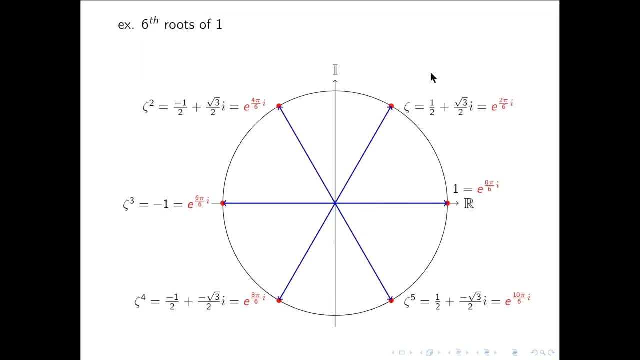 going to have a modulus of two pi k over n times i. so here's an example: i'm looking for the sixth roots of one, and so the nth roots of one are all the complex numbers, z of the form e to the two pi k over n i. but in this case n is six. so we're looking for complex numbers of the form e to the two pi k. 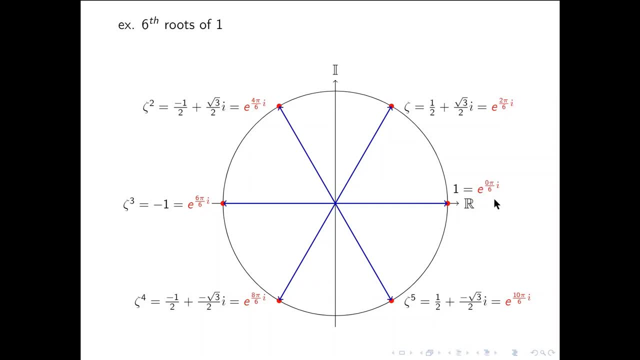 over six i. and so what if k is equal to zero? well, that's just one. one is equal to e, the two pi k where zero over six times i, right? or in other words, one is equal to e, to the zero, and one is, in fact, one of its sixth roots. one is always going to be one of its roots, all right, but what is the next? 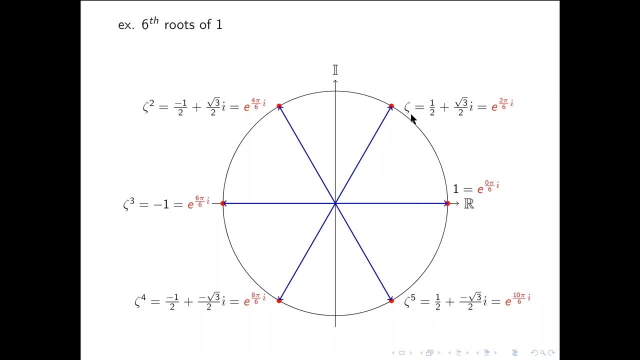 root. okay, and this greek letter is zeta. all right, so i have another one zeta, which is equal to e, to the two pi over six. i, okay, so in this case k is equal to one, because i am adding on to the argument of zero one of two pi, and then that is being divided by n, which is six. 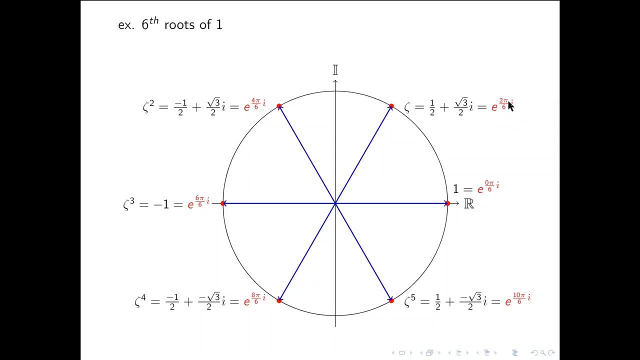 so i'm adding one, the integer multiple one, of two pi to zero, and then i'm dividing that by six. how about this one? all right, so the next root is e to the zero plus two pi times two. so k is two divided by six, or e to the four pi over six, or e the two pi over three times i, and so that is this. 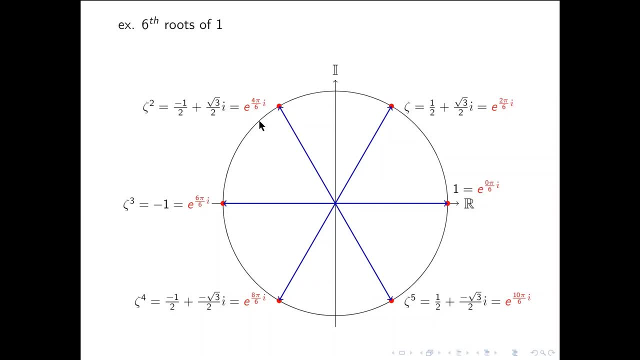 point on the complex plane and so on. you can see that for all of these, for the numerator of each of these fractions that have a six and six in the denominator, i'm just adding another integer, two pi, and you'll notice if i start right here. so this, this point here, for this complex number, is: 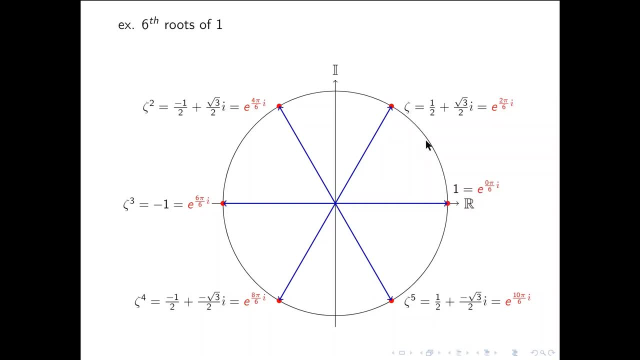 zeta, just zeta, we'll focus on that one. okay, it represents an angular distance that i'm traveling and so if i multiply by zeta, again i get here, all right, so that's the second time. then i multiply by zeta a third time, and i get here a fourth time, and i get here a fifth time, and i get here, and 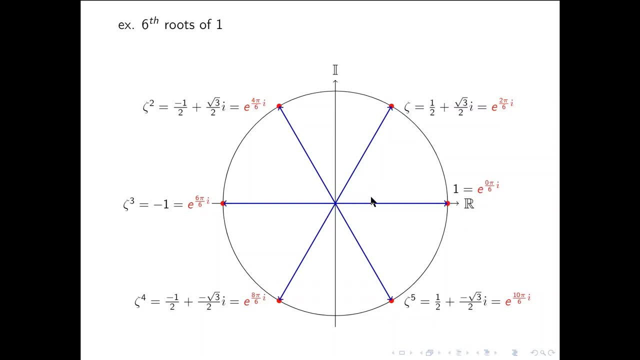 the sixth time and i get back to one. and that is of course, because when i add complex numbers or multiply complex numbers, i get back to one. and that is of course because when i add complex numbers, whether by each other or by themselves, i am adding the arguments and multiplying the moduluses. 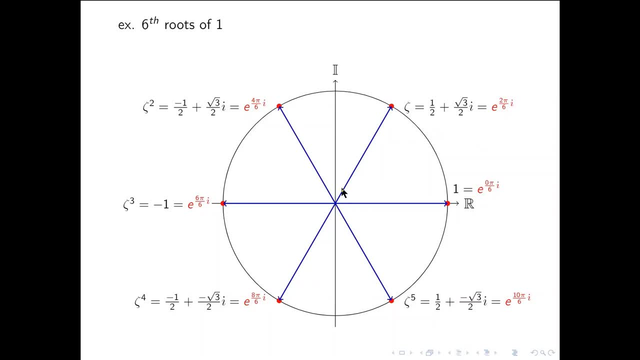 but since these are the roots of one, the modulus is one, and so when i multiply them by one another, i am keeping the modulus constant, because one times one is one and since it's the same complex number- zeta- that i am multiplying by itself, when i add the arguments, i'm adding the same argument. 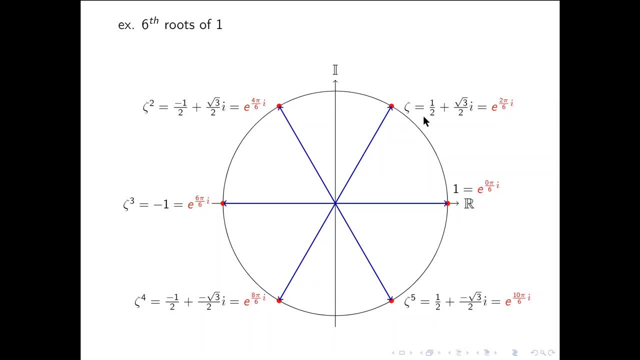 over and over again. how about for zeta squared? zeta squared is not just this sixth root of one multiplied by itself again, but it is its own sixth root of one. and so that's the same thing as well. right, if i travel this angular distance, and this should be 120 degrees? okay, if i travel. 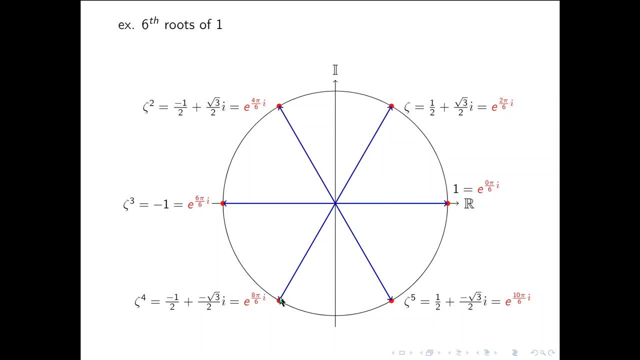 this angular distance. all right, so that is one of zeta squared, then i do two of zeta squared, i get here three of zeta squared and i get here four, and i get here five, and i get here and six and i get back to one. so, in fact, if i travel the angular distances that each of these points that are, 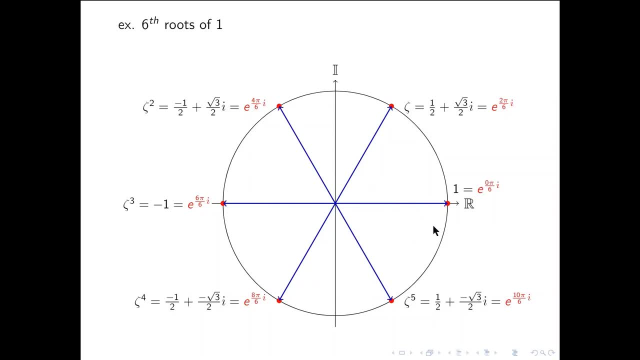 sixths around the circle describe six times. i always arrive back at one and that is why they are the sixth roots, and you can see that i get back to one and i get back to one, and i get back to one. see that there's sort of a geometric property that's arising here because of the fact that i'm 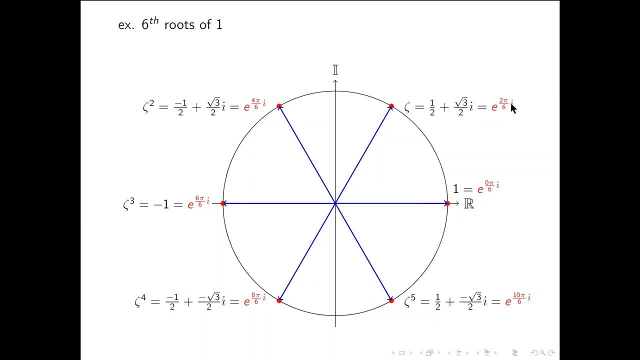 adding integer multiples of two pi to the argument of zero and then dividing by n for the nth root. okay, when i'm looking for the nth roots of one, whether they're the sixth roots or the 12th roots, whatever i'm looking for, and that is that i divide the unit circle into angular sections that have: 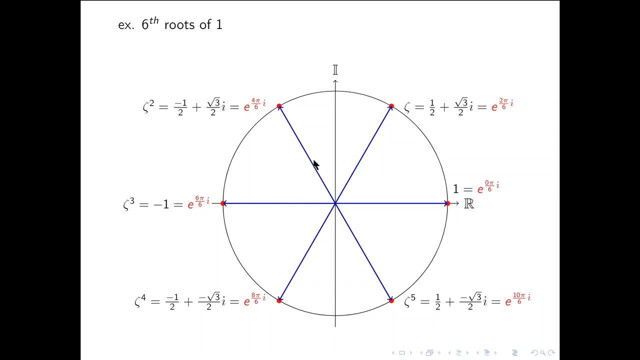 an angular distance or an angular width that is equal to sort of an nth section of the unit circle. so these are sixths, and if i were looking for an angular distance i would be looking for the twelfth roots. then i would divide the circle into twelfths and each of the points along the 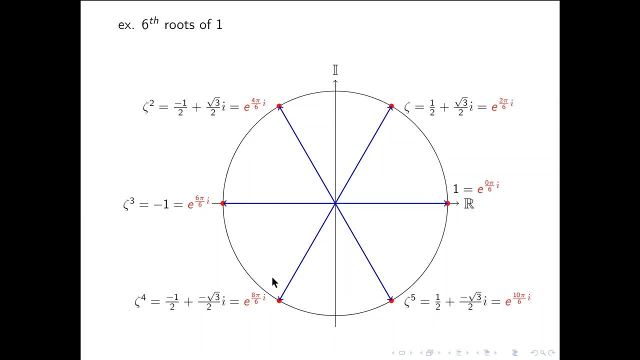 twelfths of the circle that i divide up angularly would be the twelfth roots of one in the complex plane. all right, well, that is it. i appreciate you watching this video and expect another one soon.